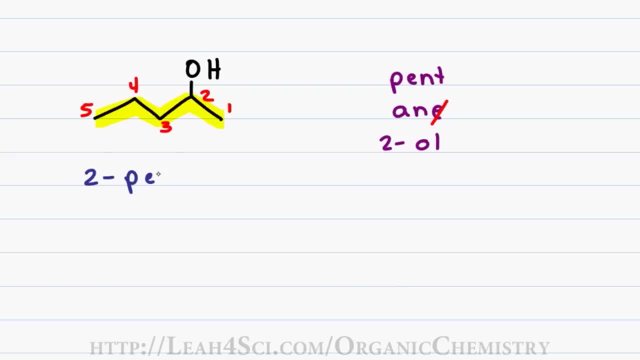 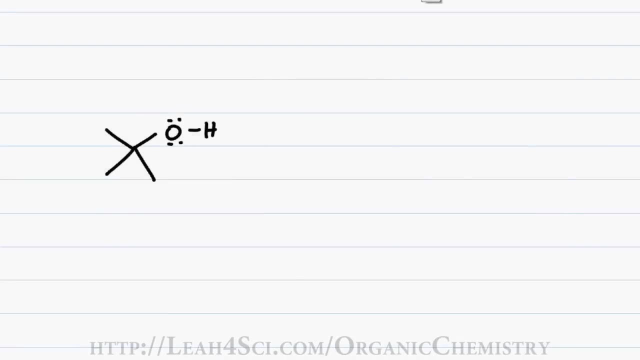 the e. This gives me a final name of 2-pentanol, where it's an instead of ane-ol. When you have a substituent on your alcohol, you still follow the same rules. where your substituent becomes the prefix and the alcohol is your suffix, You may recognize this molecule. 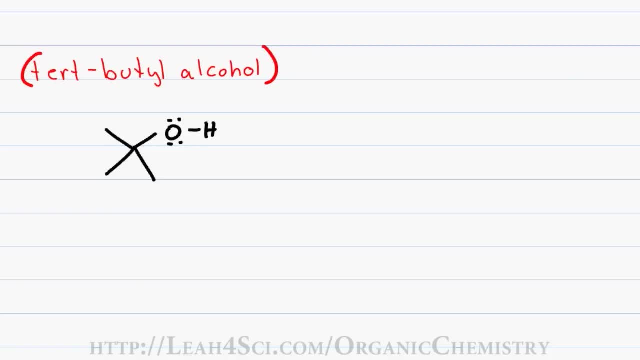 as having the common name tert-butyl alcohol, but let's see how to name it using the IUPAC rules. We'll start by identifying and highlighting our longest carbon chain- In this case it's three carbons- and numbering so that alcohol gets the lowest number. We have the option. 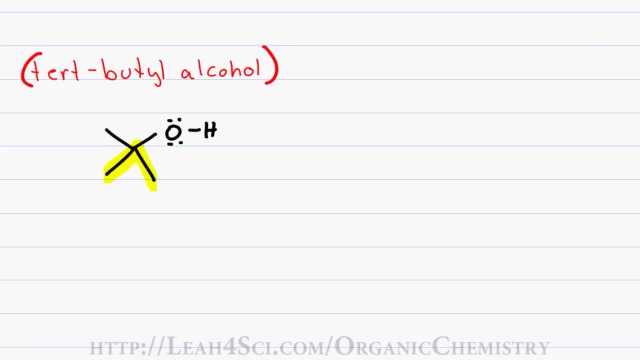 of numbering both from the right and the left, each giving oxygen a number 2.. So I'll start numbering from the left. Having three carbons in my parent chain gives me a first name of prop. Having only single bonds gives me a last name of ane, Since the alcohol is on. 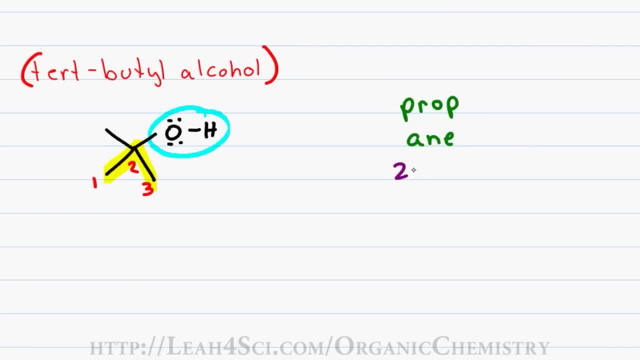 carbon 2, I have a suffix of 2-ol and since the methyl is also on carbon 2, I get a prefix of 2-methyl. Putting the name together, remember that the prefix goes first, then the first name, then the last name, then the suffix. Remember to drop the E from ane for a final. 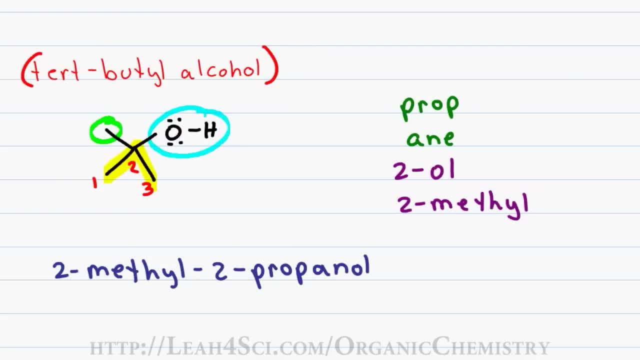 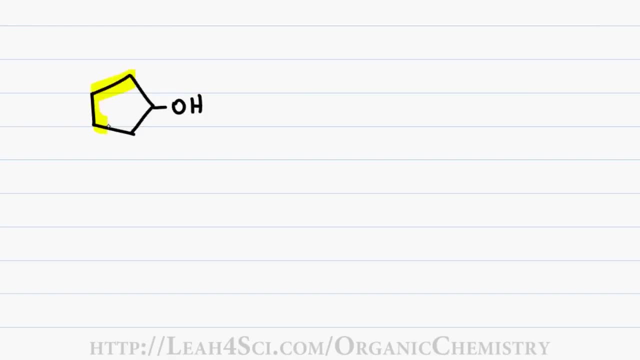 name of 2-methyl 2-propanol. The rules for naming a cyclic alcohol are just like straight chain alcohols, where you start by identifying the parent chain, In this case, a total of five carbons for a first name of pent. Given that the molecule is a ring, I'm going to 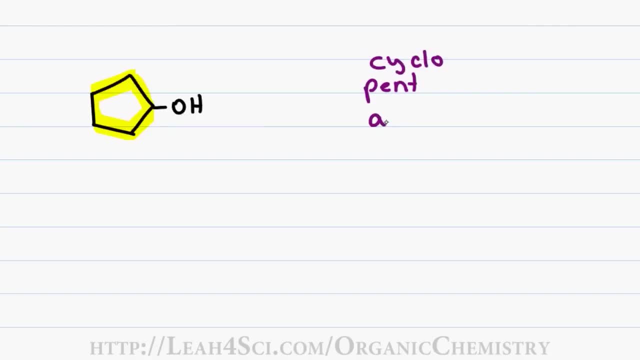 add the prefix cyclo. Only single bonds gives me a last name of ane. Since alcohol is the only group on the molecule, I give it a number 1 and then choose to go clockwise or counterclockwise, for a total of 5.. The alcohol would give me a suffix of 1-ol. However, since it's the 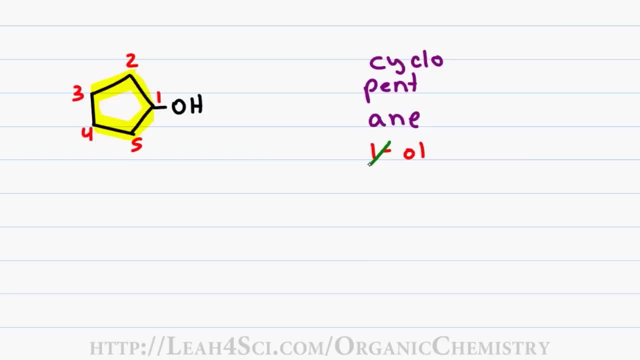 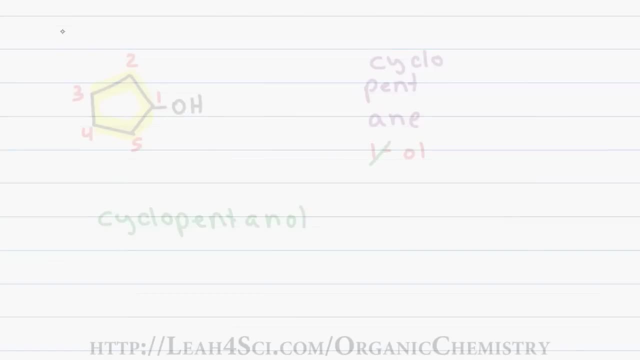 only group on the molecule. the number 1 is understood and does not have to be included. This gives me a final name of cyclopentanol. A diol is a compound that has two OH groups in the same molecule, and we'll use this as an example. My parent chain has a total of 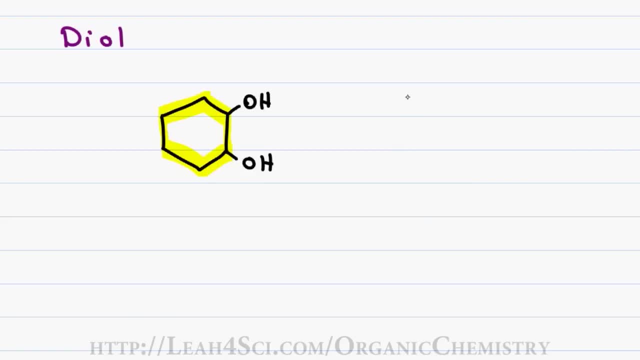 6 carbons in a ring. That gives me a first name of hex and a prefix of cyclo. Only single bonds gives me a last name of ane. Since this is a symmetrical molecule, I can choose to number from either direction, as long as one OH group gets number 1 and the second one. 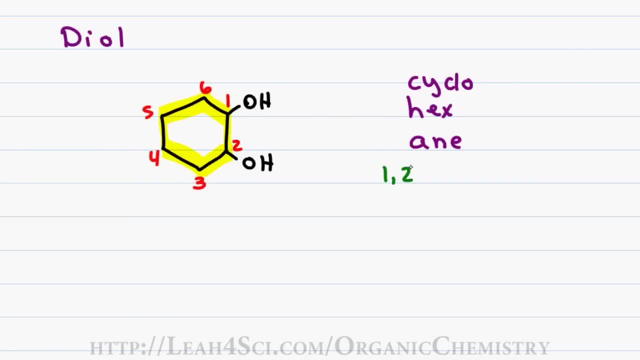 gets number 2.. I will write 1,2 to show which carbons the OH groups show up on and then put di in front of the OL to show that I have two alcohols. Putting the name together, I get 1,2-cyclohexanediol. Notice that I did not drop my E in this case, given that I have 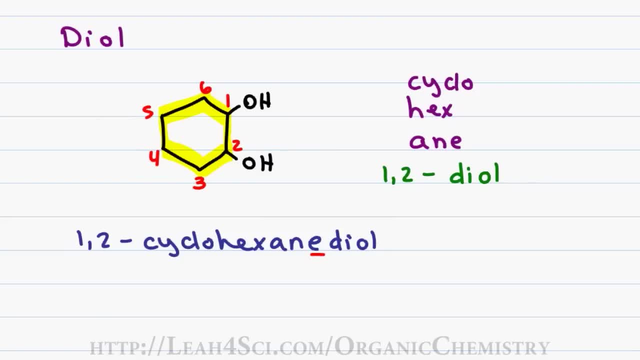 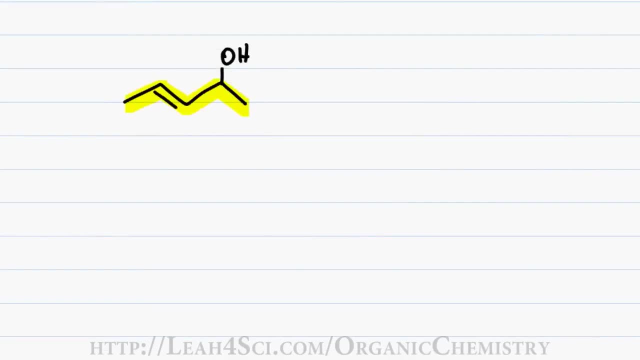 the consonant D in between two vowels. Let's try an example. with the pi bond Identifying my parent chain, I see that I have a total of 5 carbons. If I number from the right, I give my pi bond the number 2.. If I number from the left, I give the alcohol a 2.. If 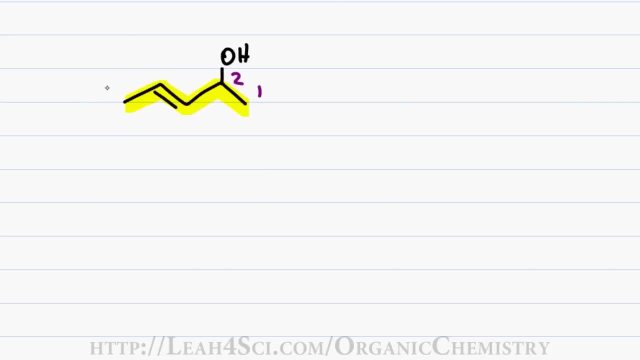 I number from the right, I get a total of 5 carbons. Since the alcohol is higher priority than the pi bond, I number from the right for a total of 5 carbons, giving me a first name of pent. Having a pi bond on carbon 3 gives me a last name of 3-ene. Having an OH. 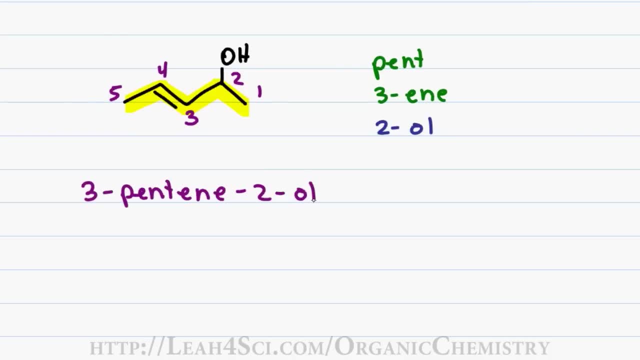 on carbon 2 gives me a suffix of 2-ol. Putting the name together, I get 3-pentene-2-ol. Notice again that I did not drop the E and that's because I have the number 2 separating the. 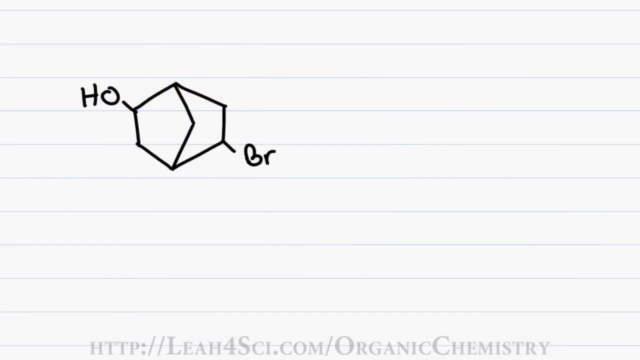 two vowels. The final problem: In this case I have two rings fused together, so I have to go back to the rules of naming bicyclic compounds. I start numbering from the bridge head closest to the OH group, since that's my highest priority, giving it a number 1, and then follow my way. 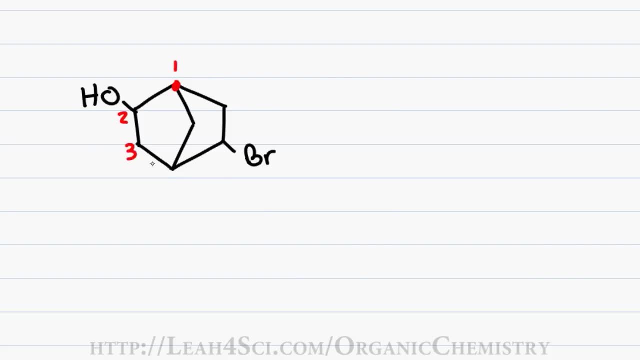 around the ring that has the OH, continuing around the ring that has the bromine and then jumping to the bridge carbon that has nothing on it. Having 7 carbons in my parent chain gives me a first name of heptane P-hep-th. having only single bonds gives me a last name of ae-n, Since I have two fused. 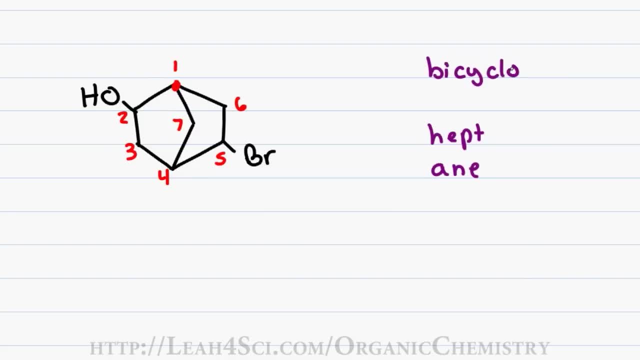 rings, I have to proceed with the word bicyclo and then I have to include how many carbons are unique to each ring in the brackets. I have two carbons unique to the ring portion, with the OH giving me 2.. I have two unique carbons to the portion with the Br giving.